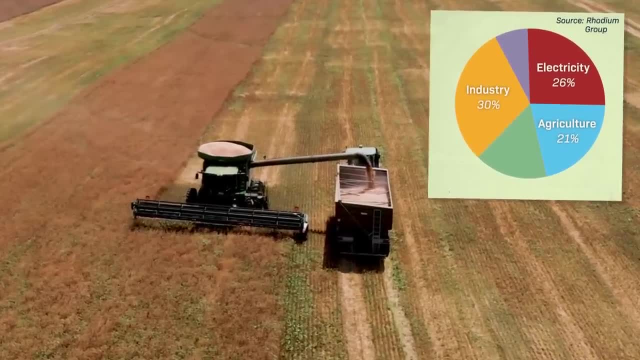 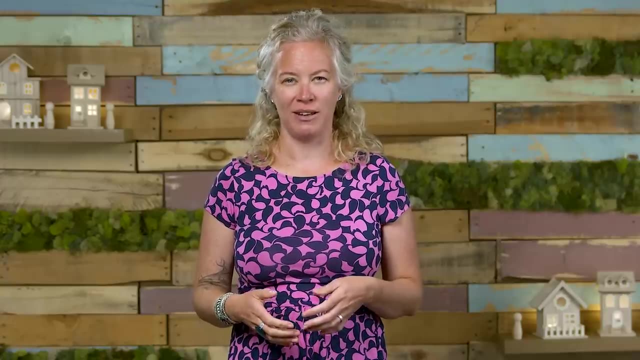 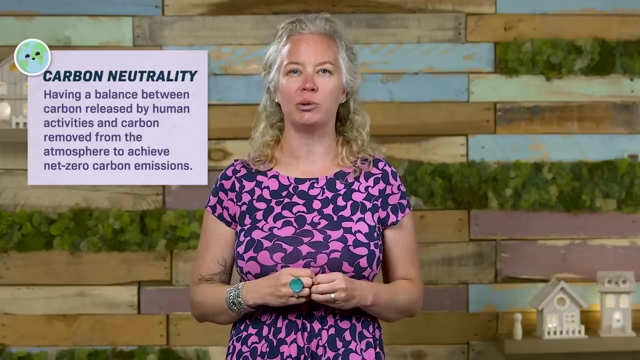 agriculture, which are often counted as their own categories when measuring fossil fuel emissions by sector. A growing number of countries are committing to becoming carbon neutral by 2050. That means reaching no net carbon emissions by both massively reducing emissions and offsetting the ones we can't avoid by scrubbing extra carbon out of the air. 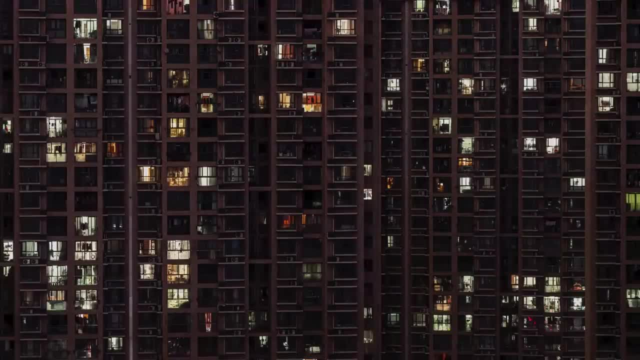 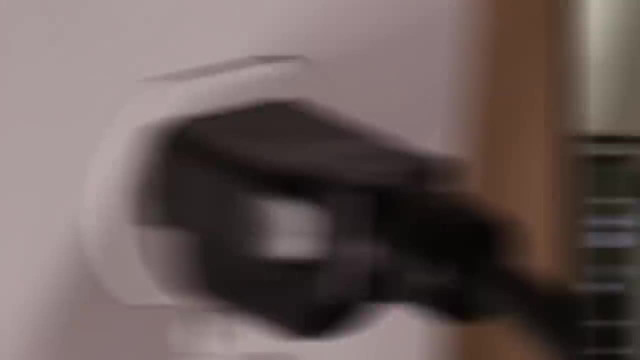 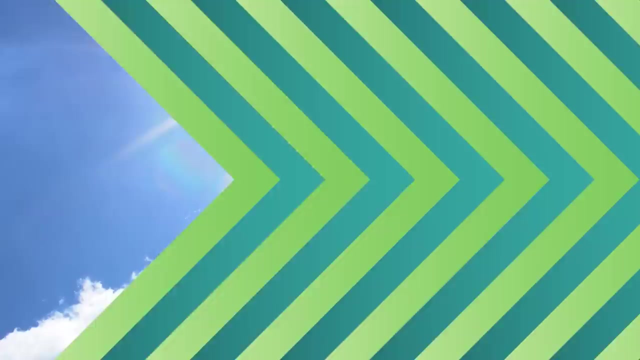 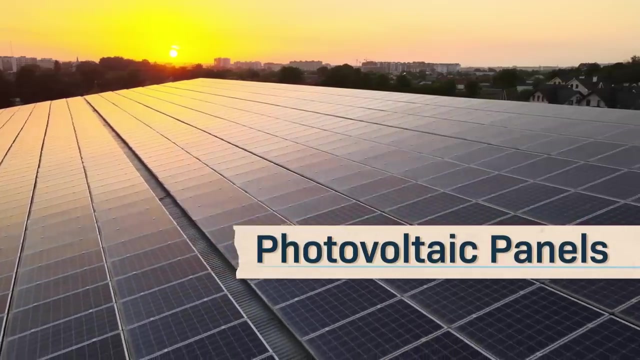 This is a challenge. We'll need to find a way to decarbonize while also meeting people's needs. The good news is we have options. Some biggies are solar and wind power. Solar power involves capturing radiation from the sun and converting it to electricity. Most often, this happens in photovoltaic panels. These panels 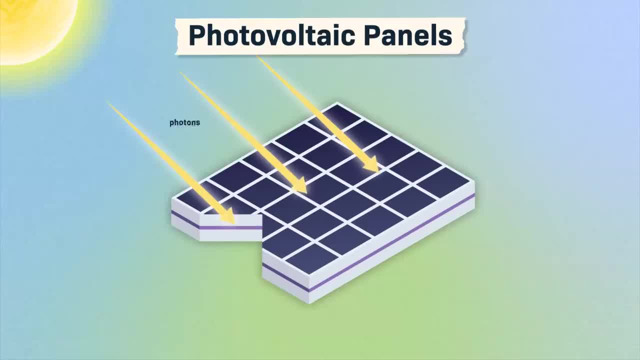 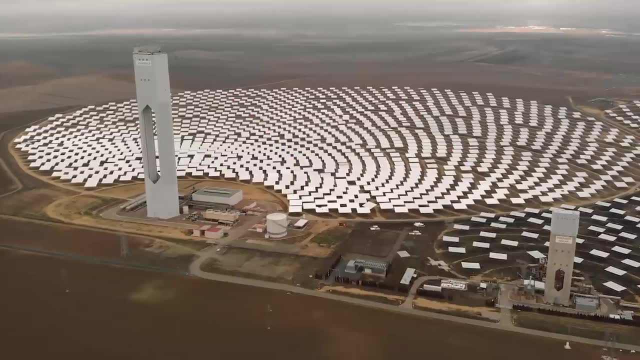 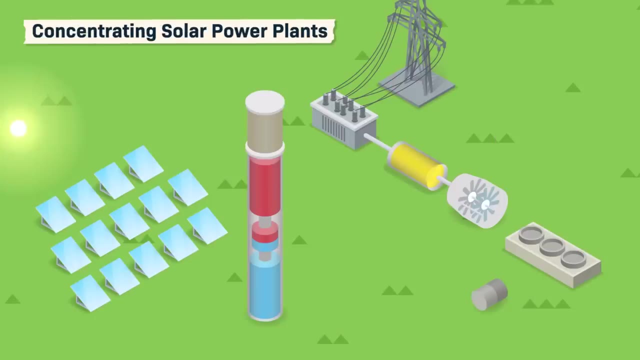 contain metals like silicon that absorb particles of light called photons and emit electrons. Those electrons are captured to form an electric current. The sun's energy can also be captured on on a large scale in what are called concentrating solar power plants. Here, instead of using a bunch of separate panels, 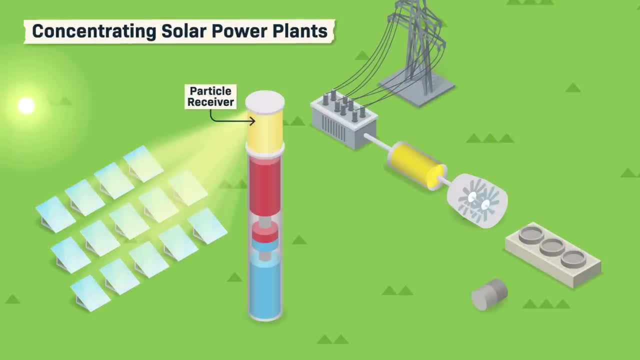 a big field of mirrors focuses sunlight onto a single receiver where temperatures can reach hundreds of degrees Celsius. It's like the coolest laser on the planet. That heat can then be used to boil water and create steam, which can turn a turbine and generate electricity. 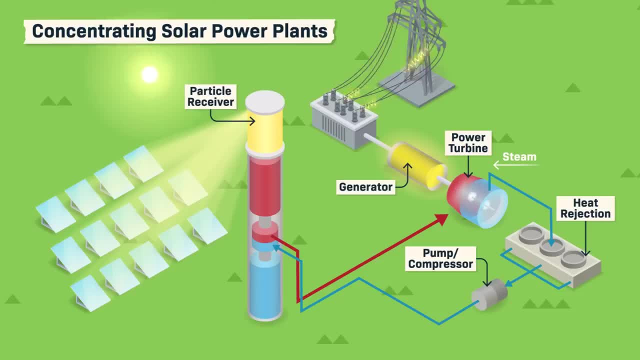 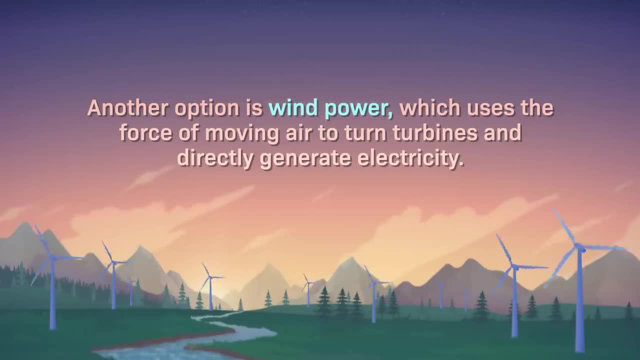 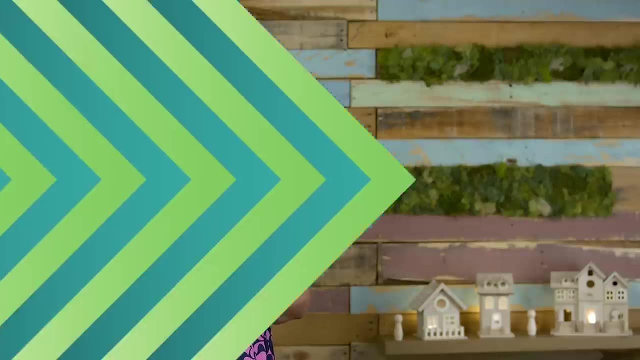 like in a fossil fuel power plant, But, crucially, it does this without releasing a bunch of carbon dioxide. Another option is wind power, which uses the force of moving air to turn turbines and directly generate electricity. There are different turbine designs for different locations. 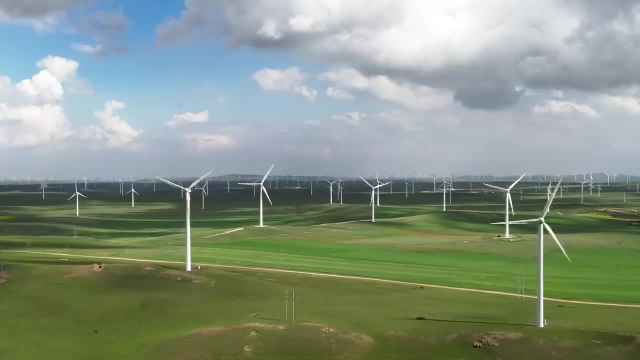 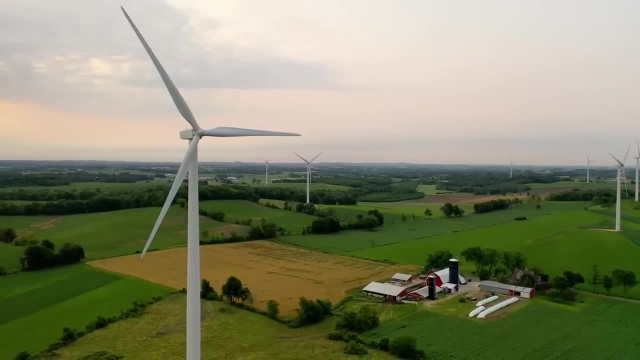 but especially if you've ever driven through a rural area, you've probably seen some of them in the wild lurking in the fields like strange high-tech crops. In the last decade, the costs of both wind and solar energy have dropped massively. 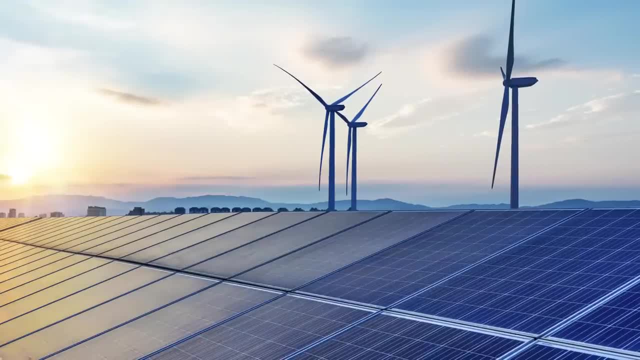 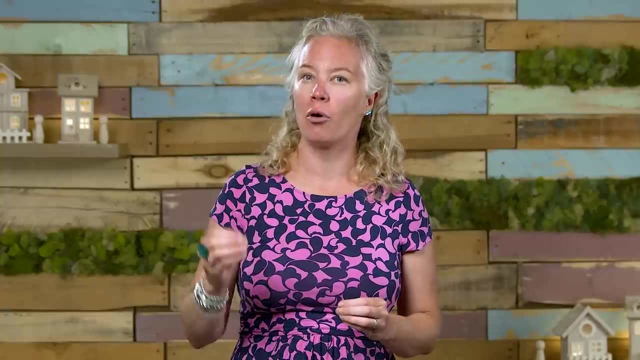 helping to make them more affordable worldwide. Because of this, wind and solar now account for about 7% of the total energy spent on the global electricity supply, And if we built and installed more panels and more turbines, that number would go up. 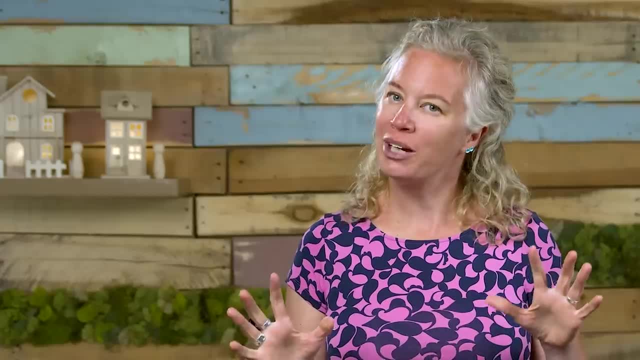 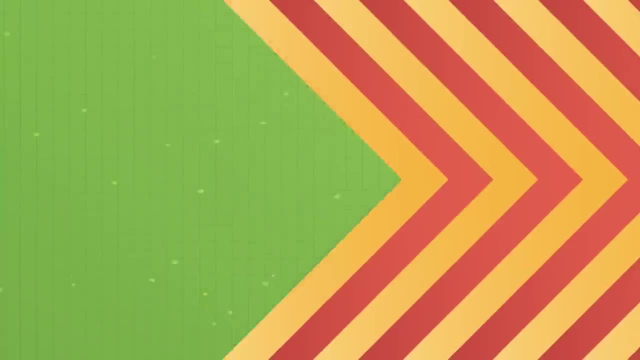 which would definitely help in reducing carbon dioxide emissions. But don't bring out the balloons. yet Scientists don't think that wind and solar could ever completely replace fossil fuel power plants. That's partly because wind and solar need a lot more space, For instance, to generate the same amount of energy. 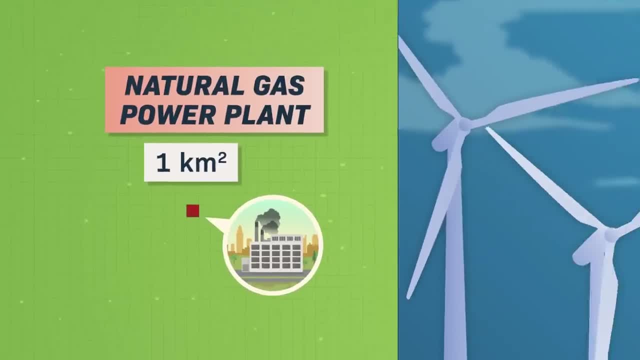 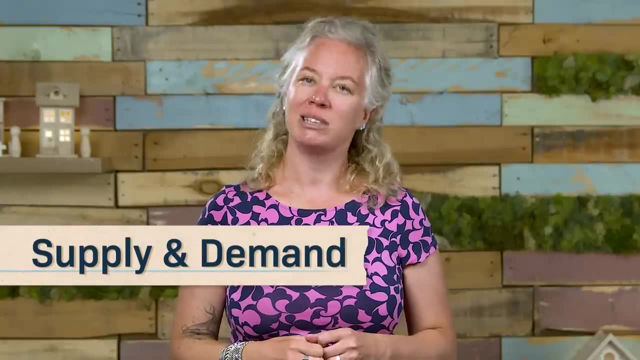 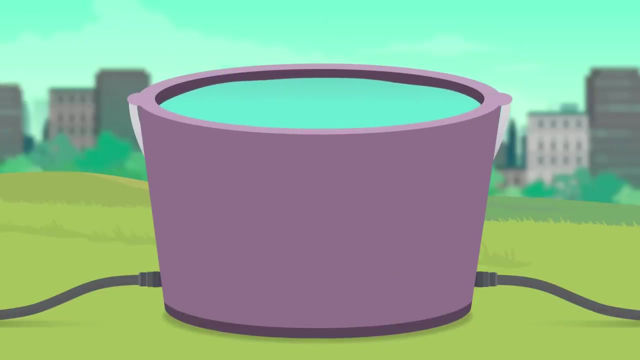 as a one square kilometer power plant. you might need 5,000 square kilometers of wind turbines, Depending on how efficient they are. But there's also another major barrier: supply and demand. Let's head to the thought bubble. Think of the electricity grid as a huge bucket of water. 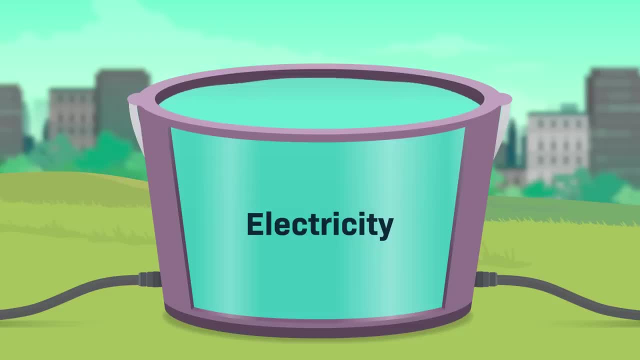 The water itself is the electricity, if you haven't guessed. And when homes and businesses need to use some of that electricity, the water flows out of the holes at the bottom of the bucket, then through the hoses, to the destination. So when you flip on the TV for a movie marathon, 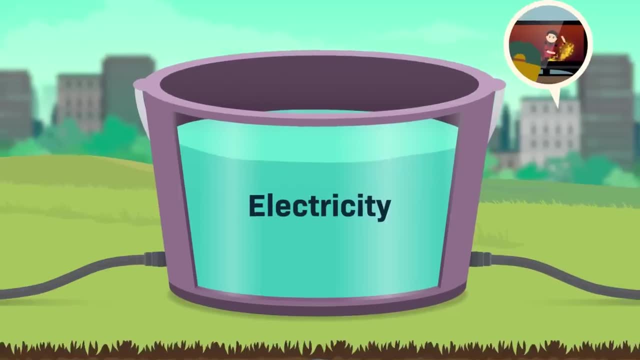 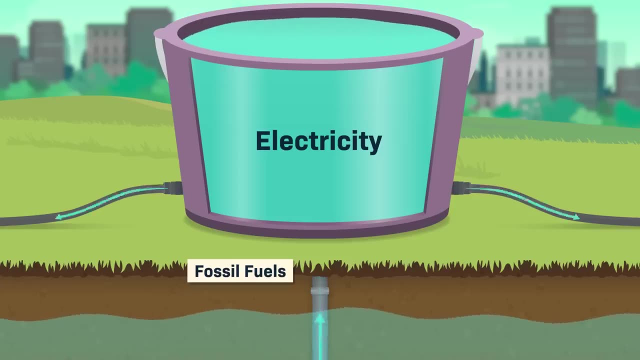 some water flows out and needs to be replaced at the top. That's where electricity generation comes in. Power that comes from fossil fuel power plants is like water pumped from underground into our bucket. Utility companies can provide a constant flow of water, which they can switch on or off. 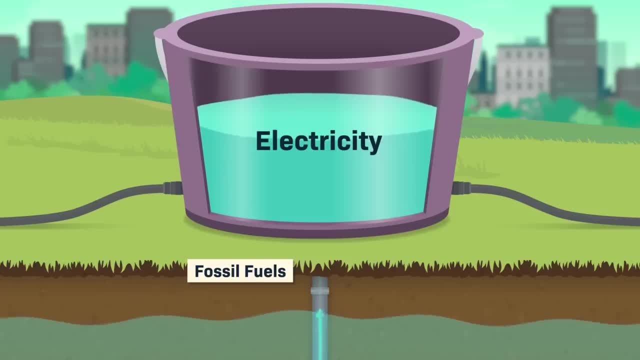 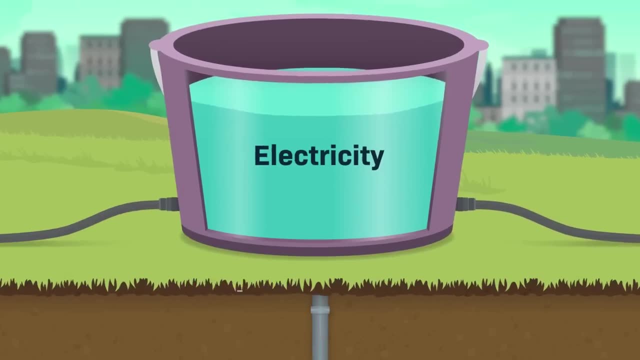 to control the amount flowing out of the bottom of the bucket, But groundwater going into the bucket, just like fossil fuels, is finite. Once it's gone, it's gone. So instead, you could opt to refill your bucket with rainwater. 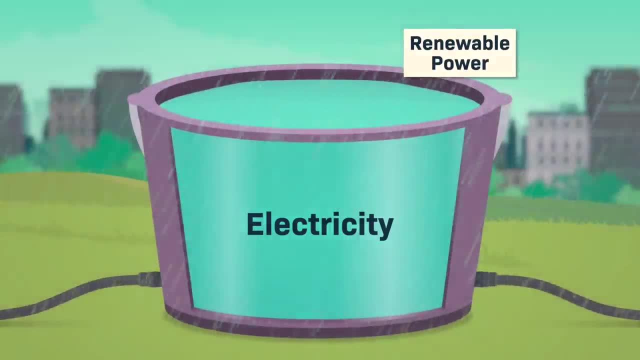 And like solar and wind power, the rain is renewable. You'll always be able to get more of it, But you have no control over when that rain falls, just like you have little control over how much the sun shines or the wind blows, as convenient as that would be. 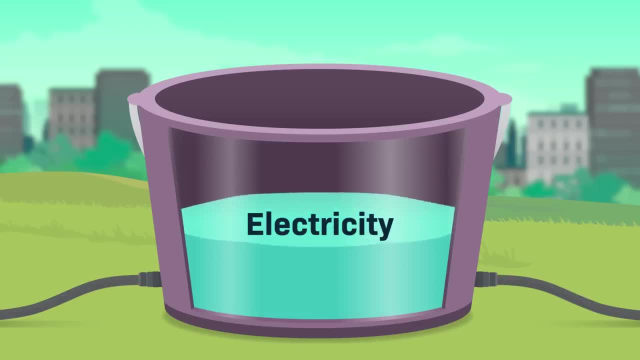 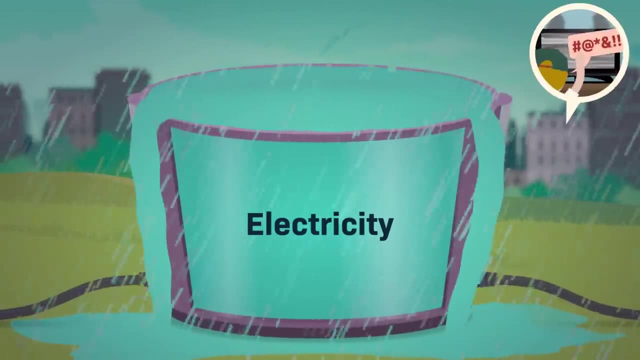 So if you relied on rainfall alone to refill your bucket, the levels could get dangerously low Or, in a big downpour, the bucket might overflow, damaging the whole system. And then there goes your plans for movie night and potentially your TV. Thanks, Thought Bubble. 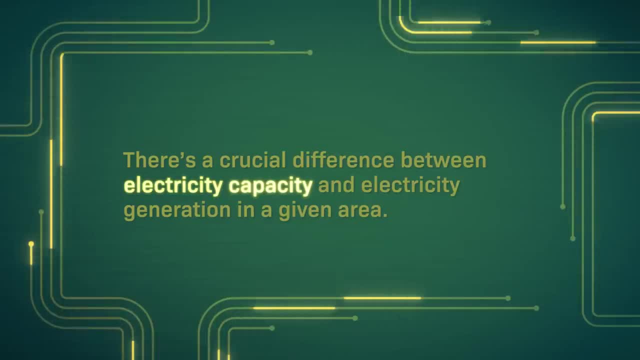 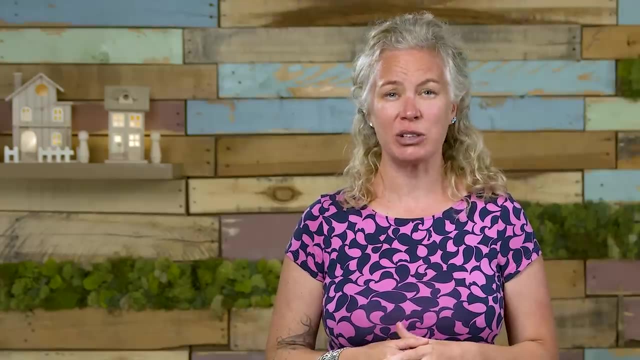 The key here is that there's a crucial difference between electricity capacity and electricity generation in a given area. In a hypothetical world with unlimited space, you might be able to install enough solar panels or wind turbines to supply the entire planet with electricity when the sun is shining the brightest. 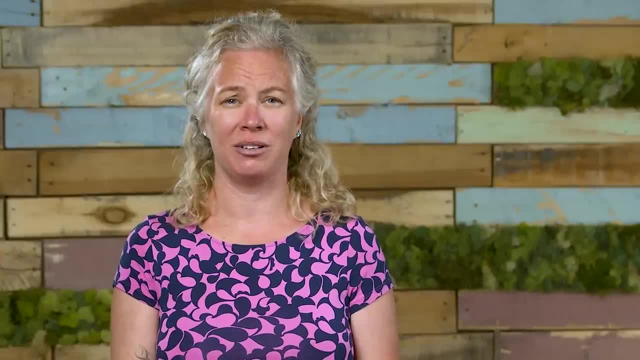 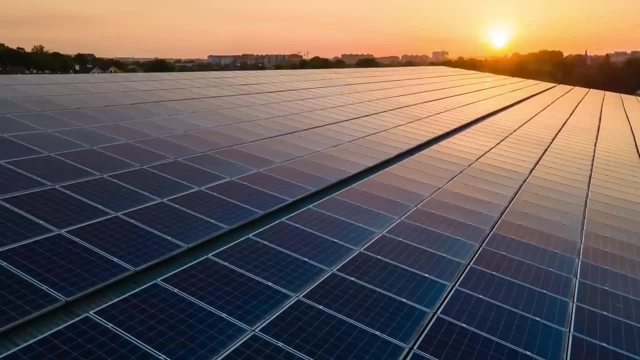 or the wind is blowing the hardest. But what happens when the sun goes down and the wind drops? Even though you might have the capacity to supply everyone's needs, the conditions outside can't generate the right amount of energy at the right time. The supply is intermittent. 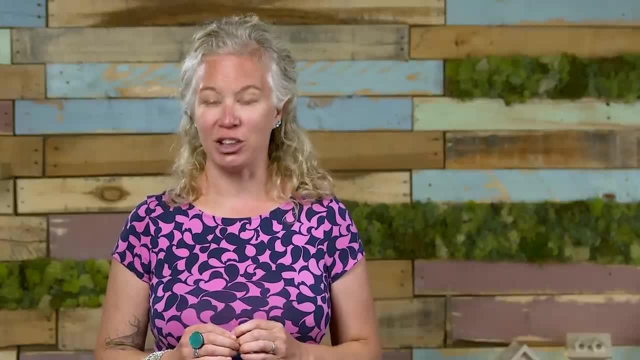 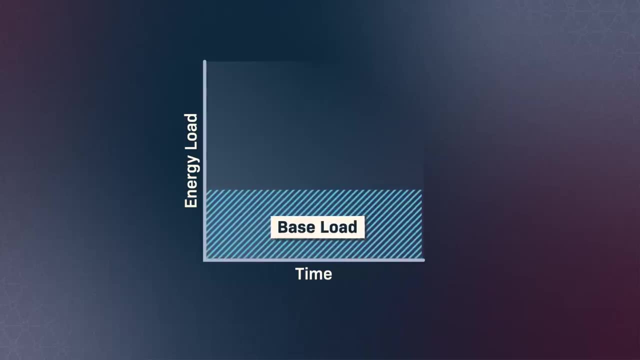 It comes and goes. Add that to the fact that our electricity usage isn't always the same either. There's always some demand for power, which is known as a baseload, But at certain times of the day and year this can increase to a peak load. 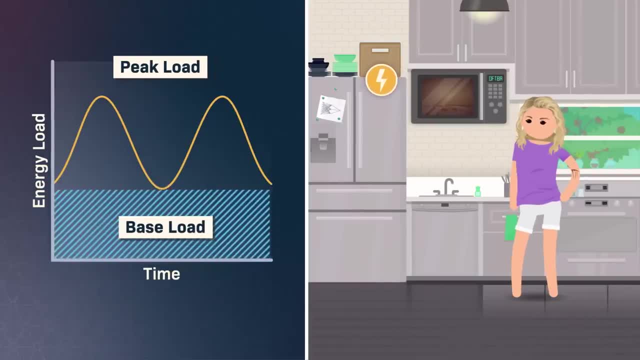 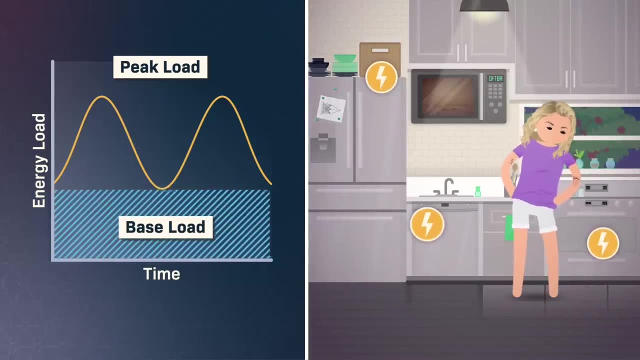 For example, say, every refrigerator in your neighborhood is always running. That's the kitchen's baseload. But in the evenings, when everyone on the block is cooking dinner and running the dishwasher and has all the lights on, the electricity grid will have to supply a lot more power than in the middle. 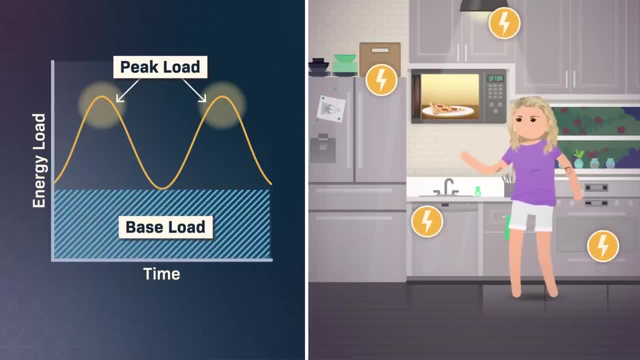 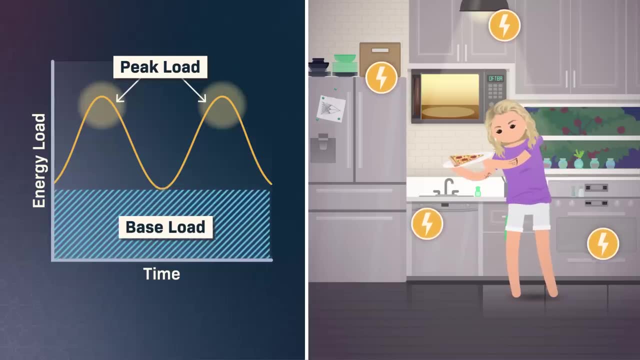 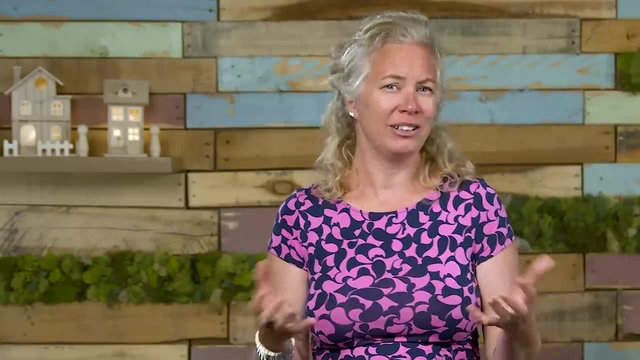 of the night, when it's just powering the fridge, or you know, the fridge plus a few people who are reheating pizza for a midnight snack. So whatever we use to supply electricity, it needs to be able to adapt to these changes And right now our demand for well power on demand. 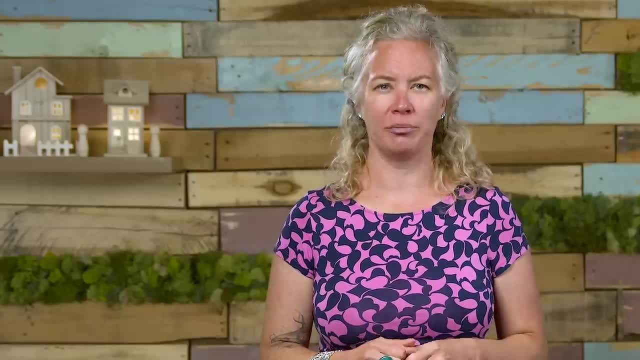 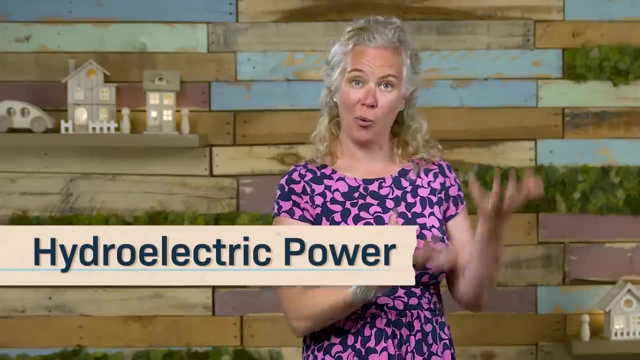 just isn't compatible with the intermittency of wind and solar power. That's where some other low-carbon options come in. For instance, hydroelectric power makes use of that old adage: what goes up must come down. Essentially, you trap huge amounts of water. 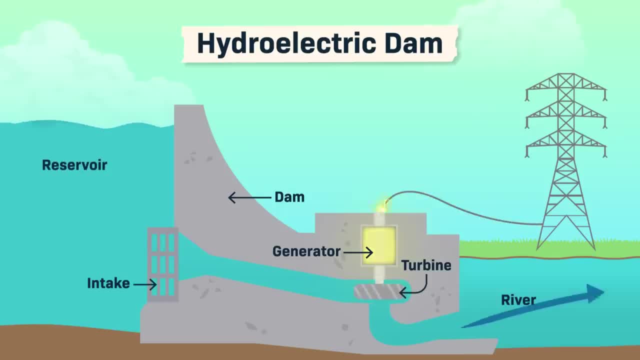 in a reservoir at the top of a hill. Then you control that flow of water downhill past turbines that spin and make electricity. Hydroelectricity is renewable, since it relies on rain and groundwater that are replaced to the natural water cycle. And after you've built your reservoir, 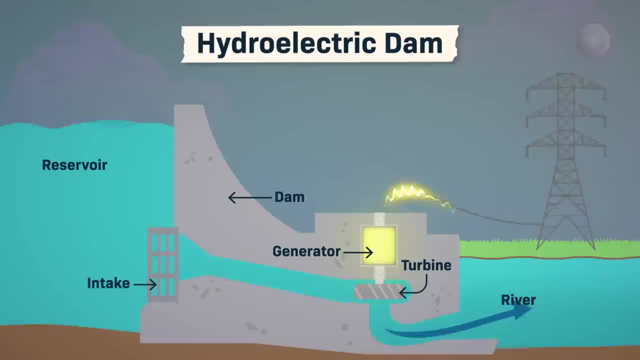 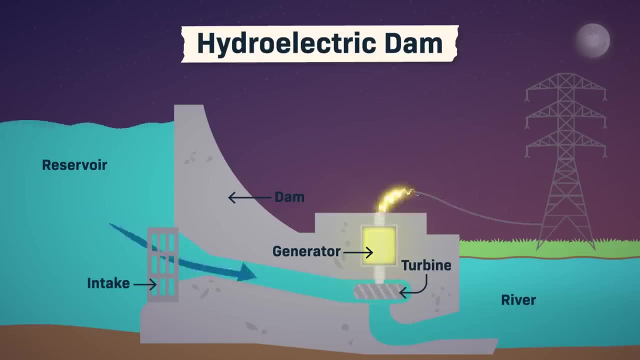 any electricity you generate is carbon neutral as well. As long as there's enough water in the reservoir, operators can also change the amount of water flowing through the facility to meet varying demand from baseload to peak load. Right now, the biggest hydroelectric facility. 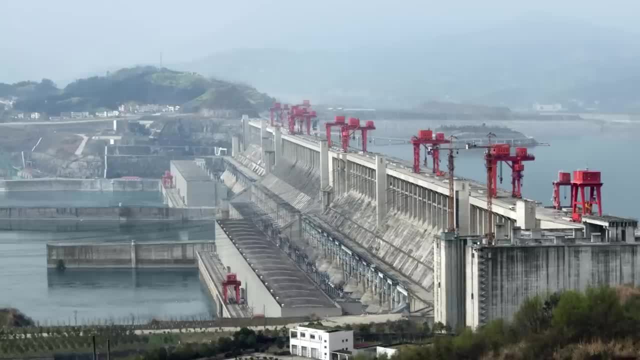 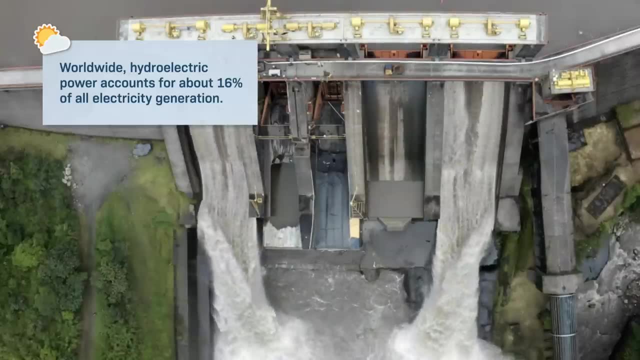 in the world is at the Three Gorges Dam in China In 2021, it generated enough energy to hypothetically power a small country like the Netherlands. Worldwide, hydroelectric power accounts for about 16% of all electricity generation, But maybe hold the confetti cannons. 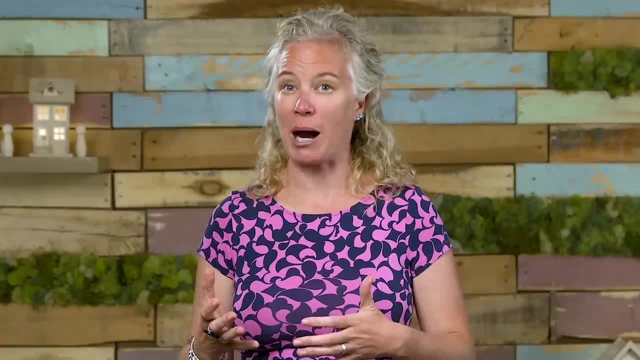 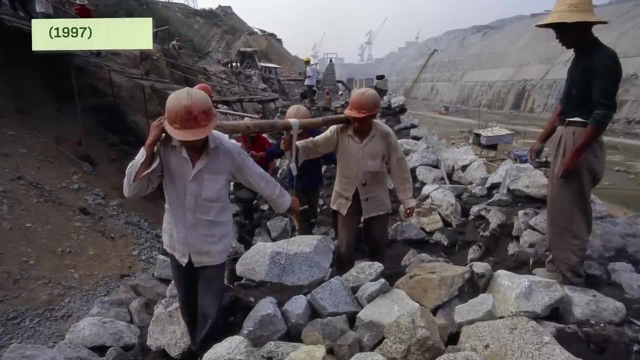 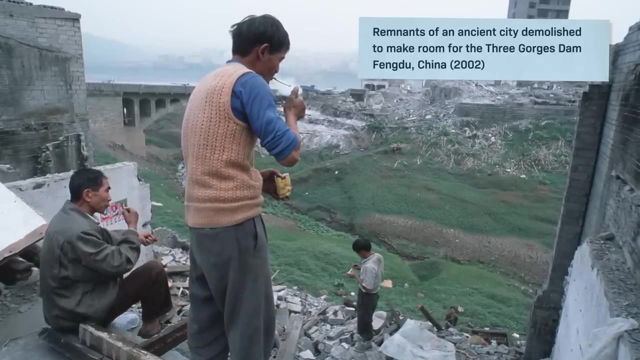 because it's not all good news. Building a reservoir capable of powering cities comes with serious environmental and economic consequences. Three Gorges took nearly 20 years to build and cost at least $28 billion. More than 1.3 million people also had to be moved. 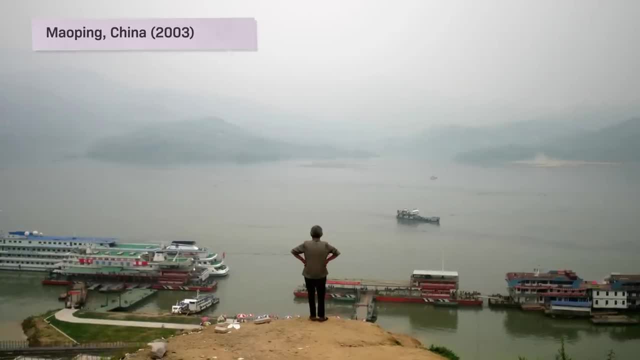 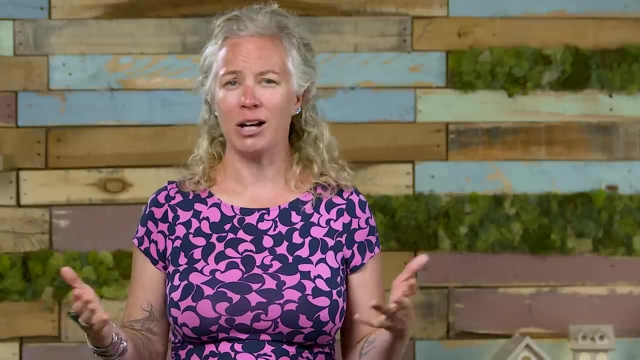 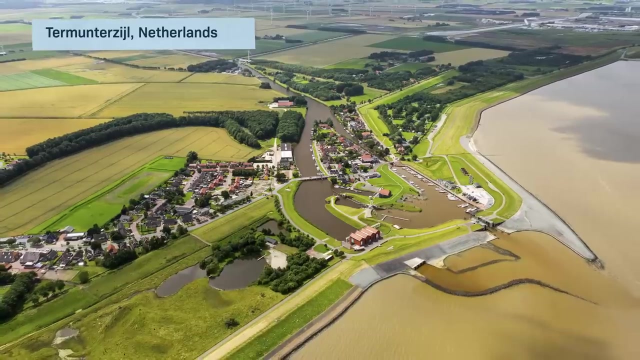 from their homes, and the Yangtze River valleys were submerged more than 600 kilometers upstream, destroying huge swaths of the natural environment. Also, hydroelectric plants only really work when you have plenty of water and plenty of drop. Realistically, a flat country like the Netherlands- 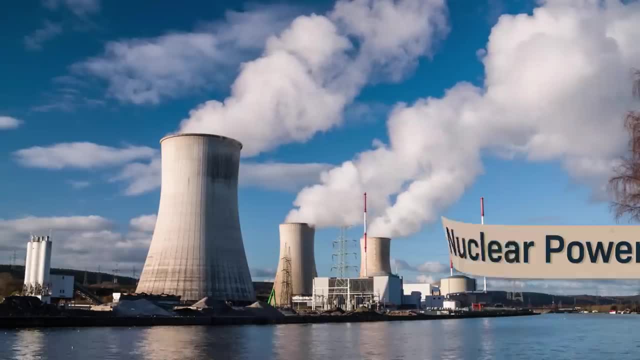 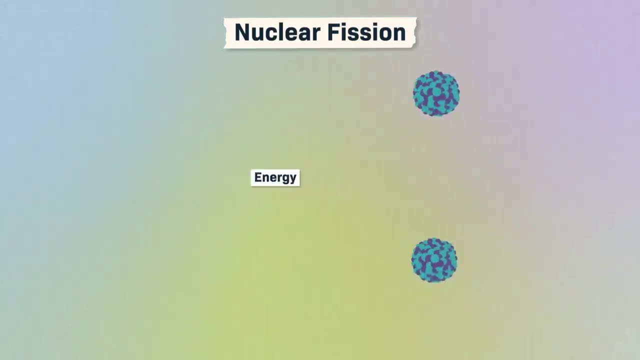 could never hope to power itself hydroelectricly. So another alternative, and one that can be a bit more flexible, is nuclear power. When you hit a large atom of uranium with another particle, the uranium undergoes nuclear fission. It breaks down into other elements while releasing heat. 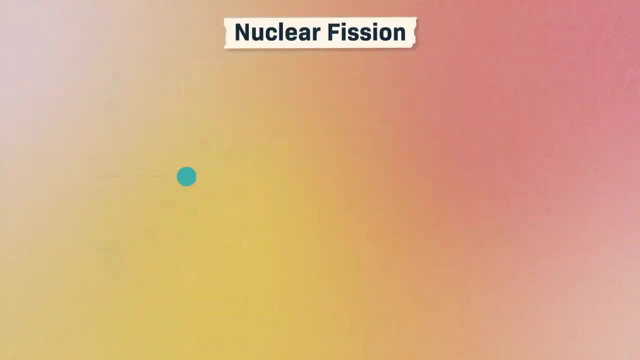 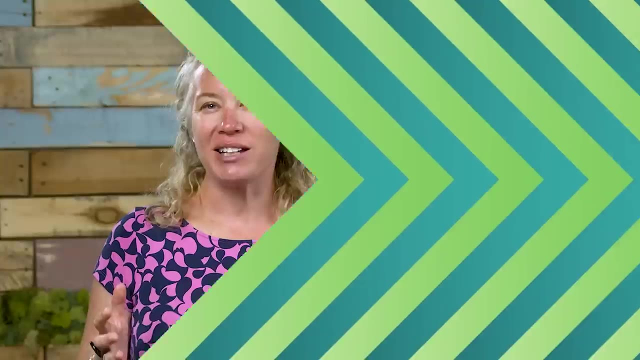 By harnessing that fission in a controlled chain reaction, the generated heat can be used to create steam and turn a turbine, just like in a fossil fuel power plant. The benefit here is that nuclear fission doesn't release any carbon, and by carefully tweaking the amount of fission, 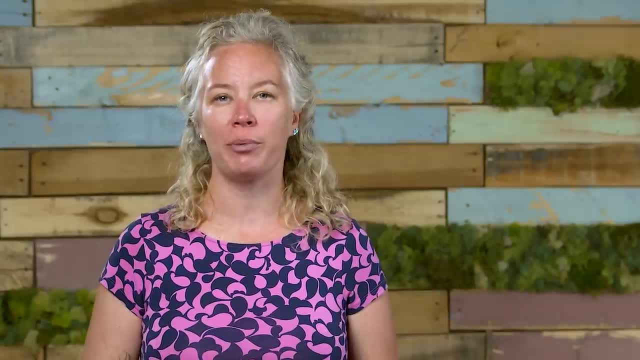 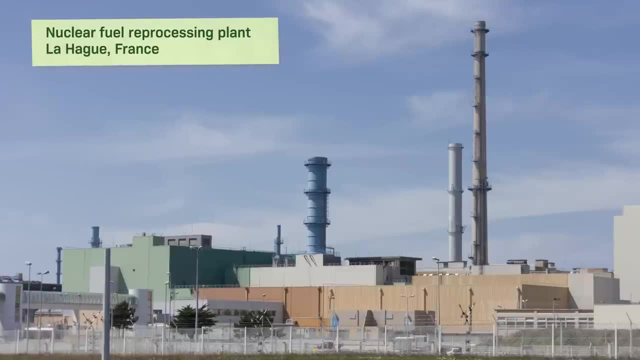 the plant can easily ramp up production to meet peak demand. Now, uranium fuel itself isn't renewable, so there's only a limited supply. But the next generation of nuclear plants is finding ways to make it last longer by using one of the leftovers from uranium fission. 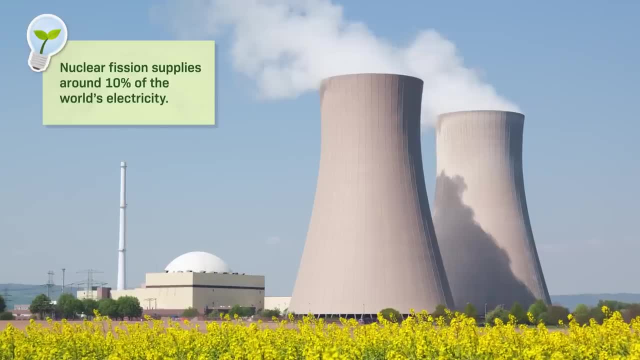 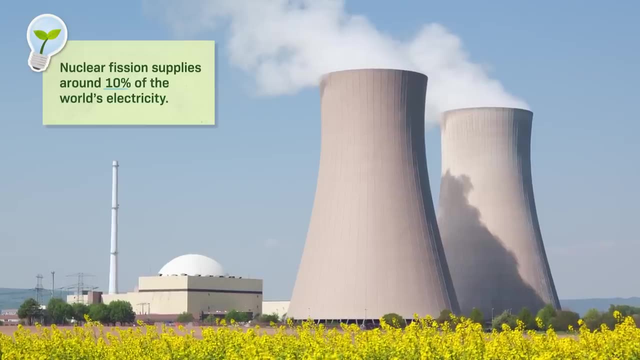 to make even more heat after round one. Right now, nuclear fission supplies around 10% of the world's electricity and since it's so flexible and scales up so well, it could supply more. But there are significant benefits. Challenges: 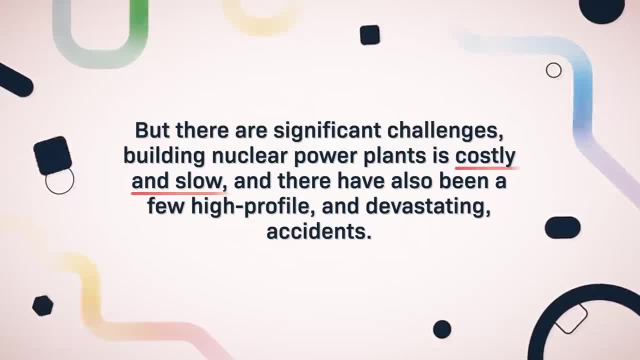 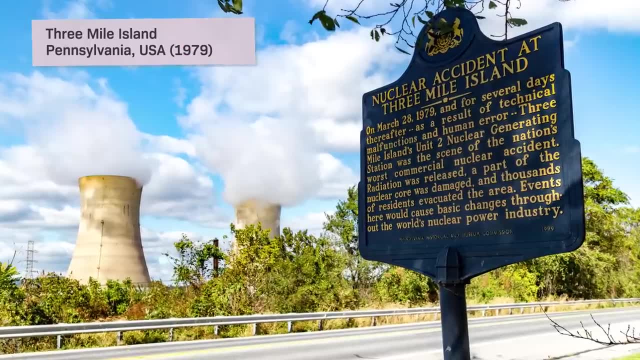 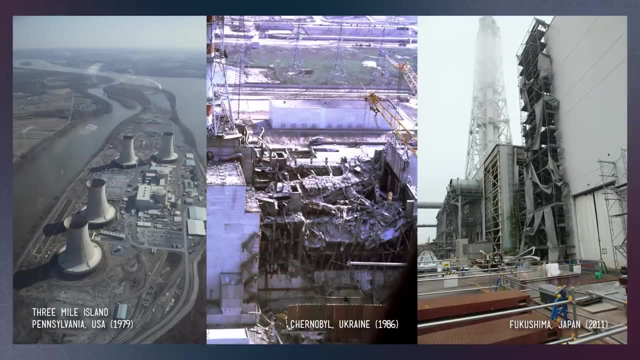 Building nuclear power plants is costly and slow, and there have also been a few high-profile and devastating accidents Throughout the years. power plants at Three Mile Island, Chernobyl and Fukushima all made headlines when their dangerously radioactive insides leaked outside. 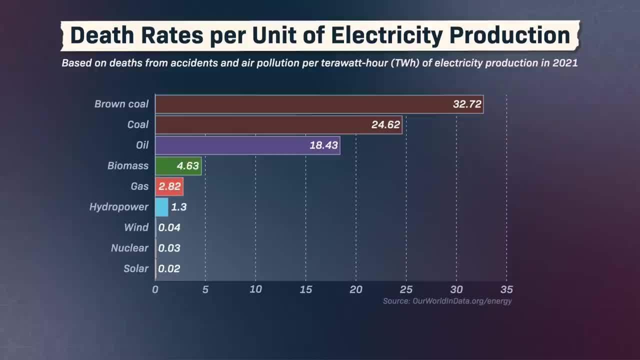 In reality, far more people have been killed by air pollution from fossil fuel power plants than nuclear accidents, But there's still a level of risk not everyone knows. And there's one that's comfortable with: Solar, wind, hydroelectric, nuclear. 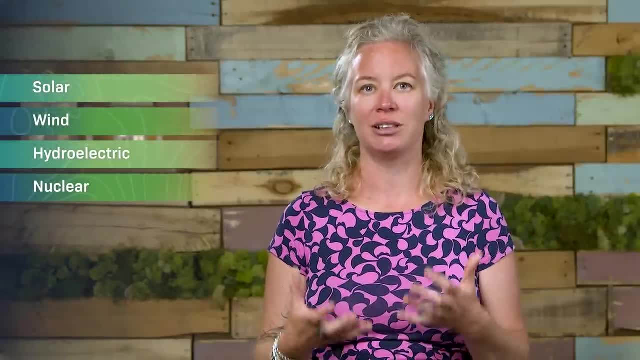 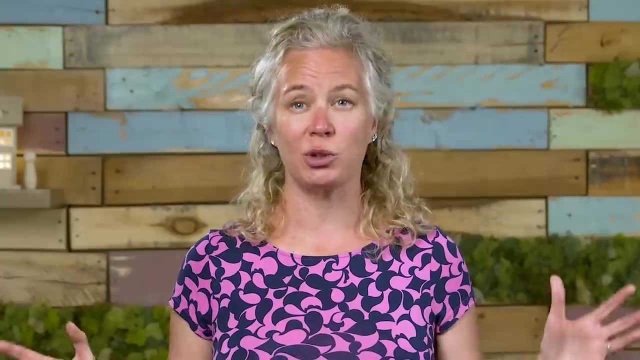 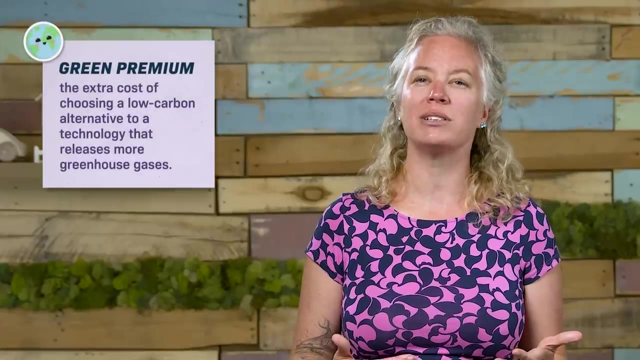 The point here is that there's not going to be a single solution to completely decarbonizing our electricity supply. It's going to take a variety of technologies and none of these transitions will be cheap, Compared with fossil fuel sources. all low-carbon options come with what's known. 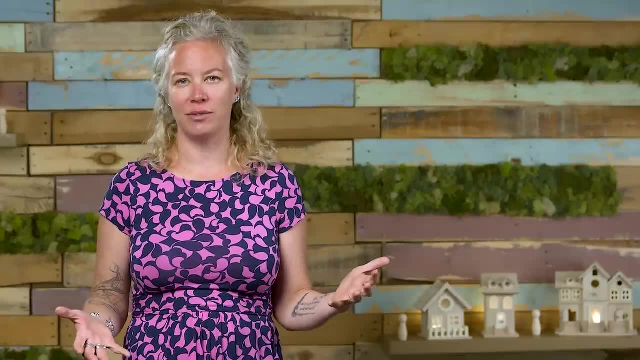 as a green premium. Over the years, many countries have done what they can to keep the price of fossil fuels low in order to boost. to keep the price of fossil fuels low in order to boost. to keep the price of fossil fuels low in order to boost. their economies and technological development. They've tapped into whatever fuel reserves they have nearby and provided tax cuts and subsidies to allow companies to produce and use that fuel cheaply. That means any new technology that doesn't use fossil fuels seems artificially expensive, even while the resources themselves 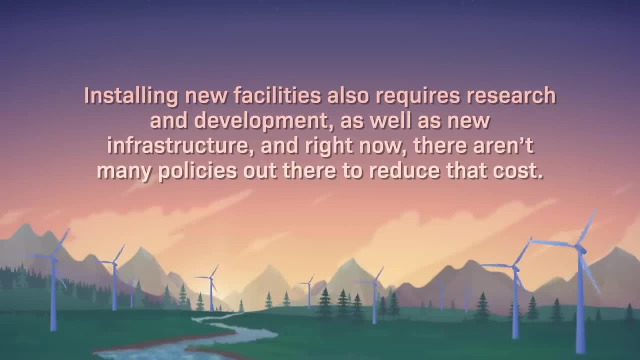 like sunlight and wind, might be free. Installing new facilities also requires research and development, as well as new infrastructure, And right now there aren't many policies out there to reduce that cost. These are not insurmountable challenges, though. 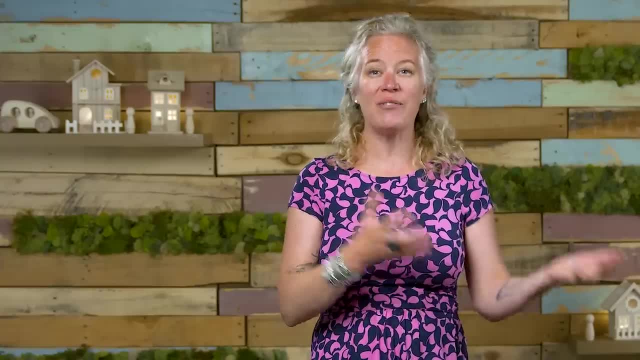 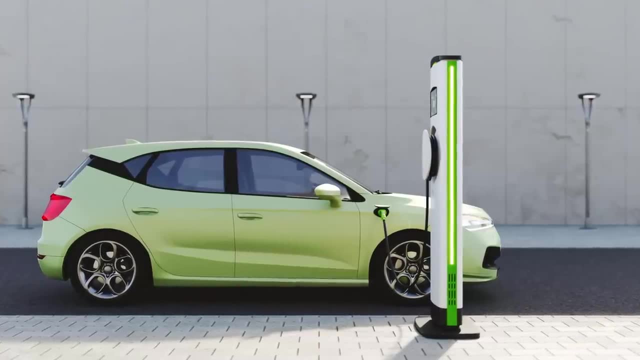 The incredible thing is that if we can decarbonize electricity, it'll have an impact on the other major industries that currently release greenhouse gases. New generations of vehicles can be fueled by carbon-free electricity instead of guzzling tankfuls of gas. 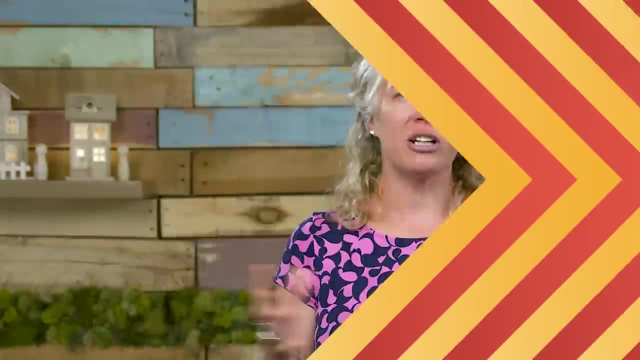 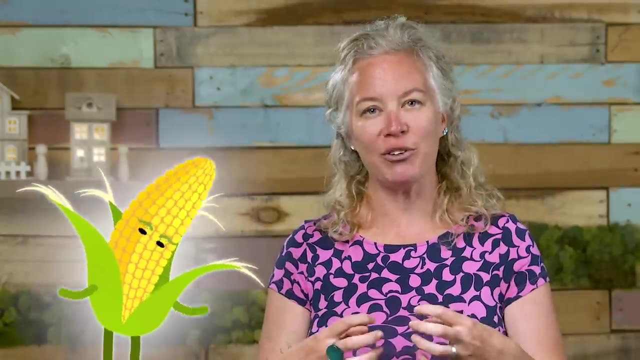 And homes can be heated efficiently without emitting carbon dioxide. Decarbonizing electricity would even help the agricultural industry, not by electrifying the crops somehow, but by powering everything that goes into growing them. We're talking electrifying the crops, electrifying tractors, pumps and watering systems. 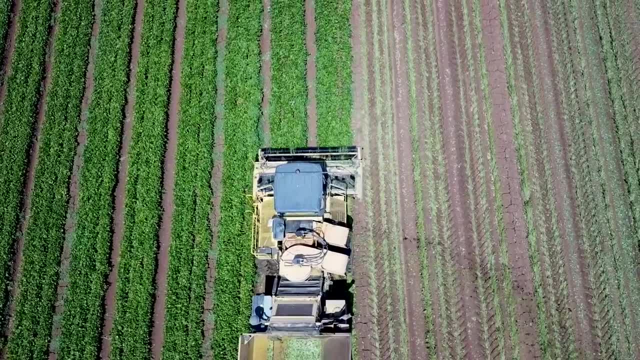 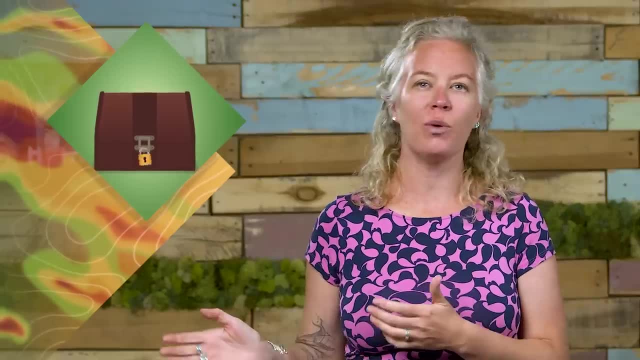 the machines that pick your green beans, heavy equipment that currently runs on fossil fuels, And for the emissions that are left. researchers are looking into ways to capture the excess carbon and lock it away where it can't cause further warming, So decarbonizing our electricity supplies. 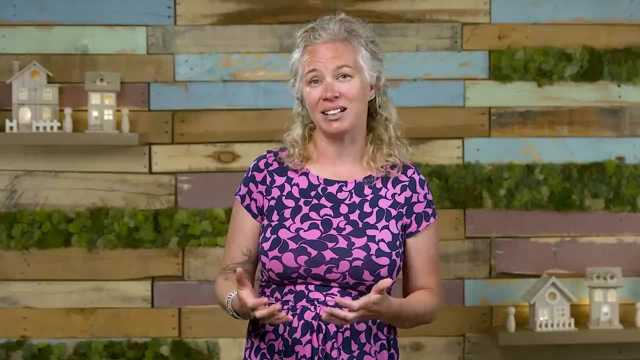 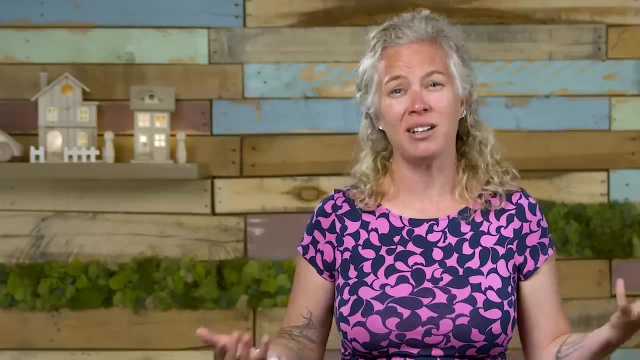 won't solve the climate crisis by itself, but it can take us a good way in that direction. Someday soon, the electricity that powers your internet or your midnight pizza might come from something like solar or hydroelectric power. In fact, it might already. 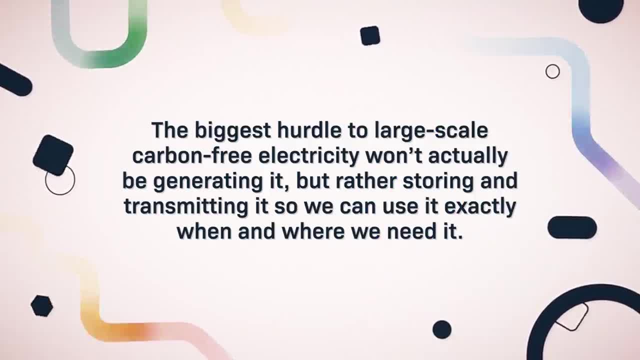 That being said, the biggest hurdle to large-scale carbon-free electricity won't actually be generating it, but rather storing and transmitting it so we can use it exactly when and where we need it. In other words, we need to seriously improve our water buckets. 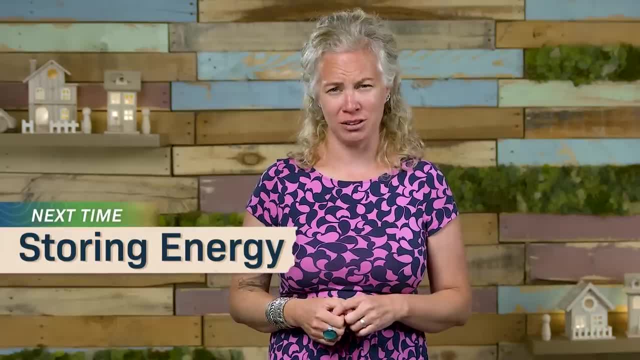 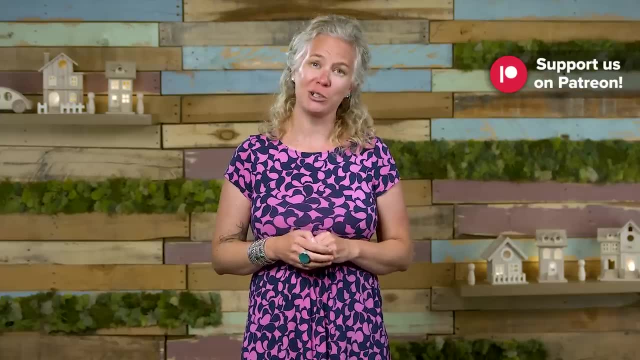 We'll explore how we do that and why it's harder than you might imagine next time. Special thanks to John Lee, this episode's mac and cheese caterer. John, we're still talking about the cool backflip you did into the swimming pool of macaroni.